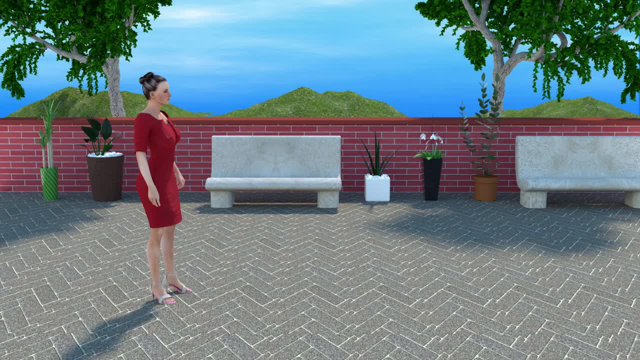 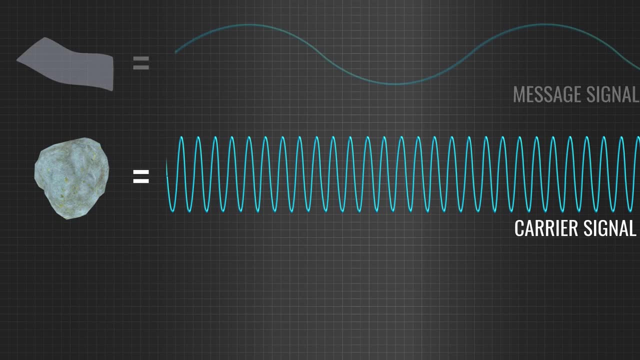 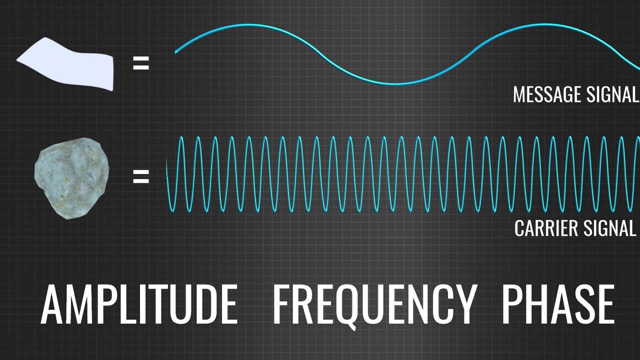 This is exactly how we do modulation. a stone modulation uses a high-frequency signal known as a carrier signal. As we know, any signal has three basic properties – amplitude, frequency and phase In the modulation process. one of the properties of the carrier signal is varied in accordance. 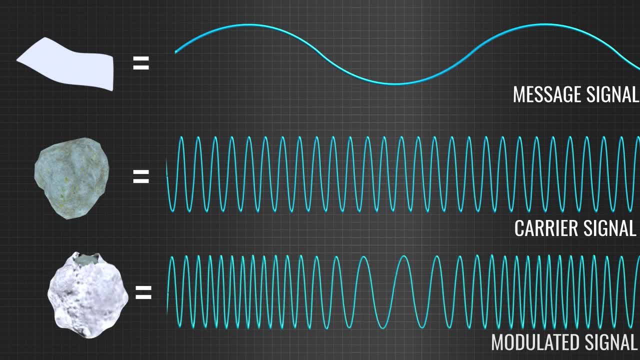 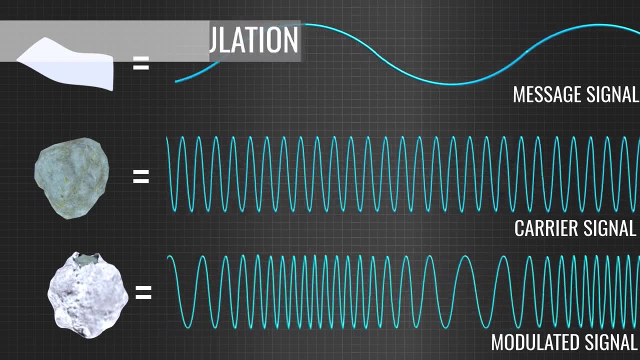 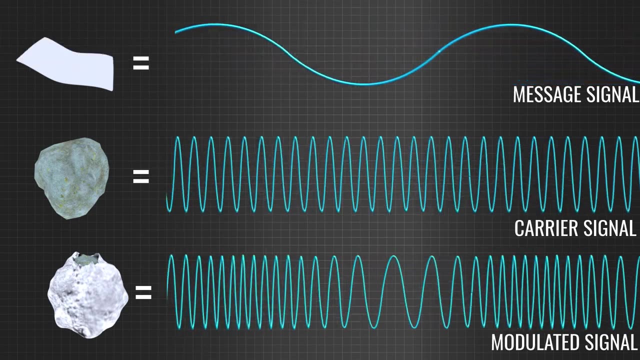 with the message signal. For example, the frequency of the carrier signal is varied according to the amplitude of the message signal. This technique is known as frequency modulation. Please note that the frequency of a carrier signal is always high, which means the modulated. 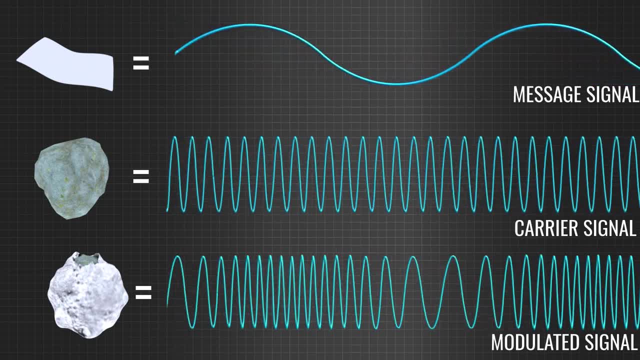 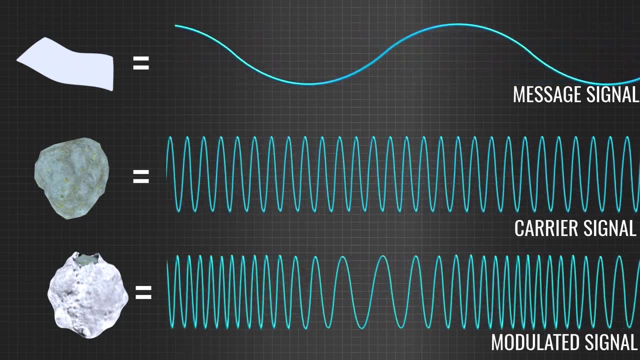 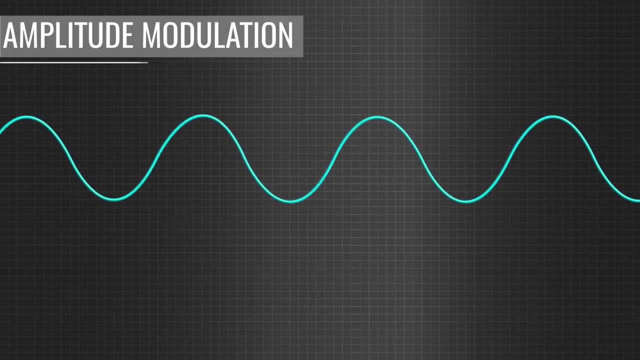 signal is also of high frequency and energy. The value of the original signal can be easily retrieved from the frequency of the modulated signal. In the same way we can also achieve amplitude modulation. Here the amplitude of the carrier signal is varied based on the value of the message. 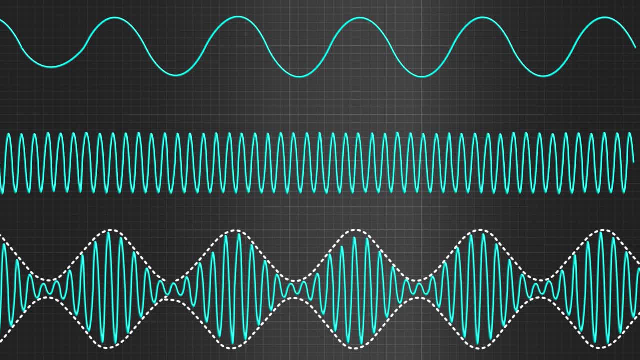 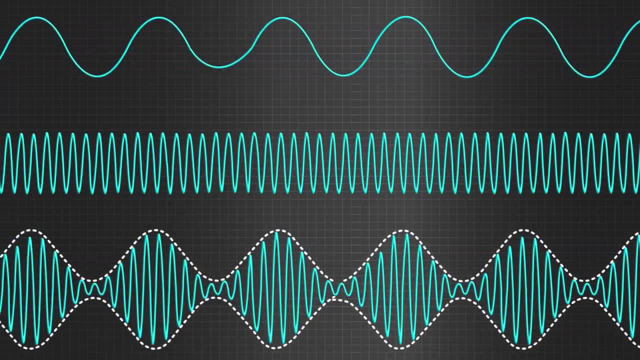 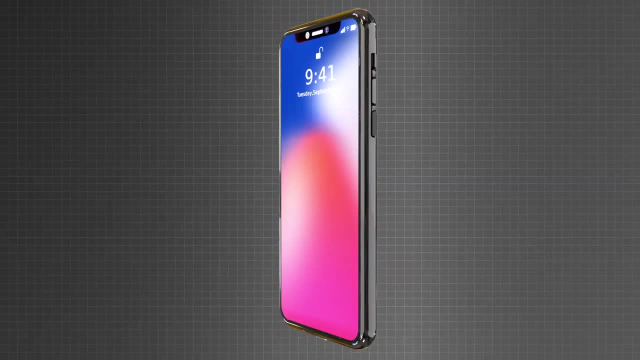 signal. The modulation techniques we have discussed so far have all been analog types. however, they are already obsolete. Analog modulation is susceptible to noise, which degrades the quality of signals, And, moreover, in today's electronic instruments, all operations are carried out in digital. 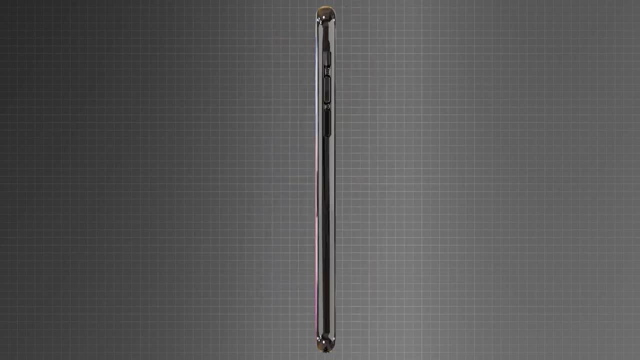 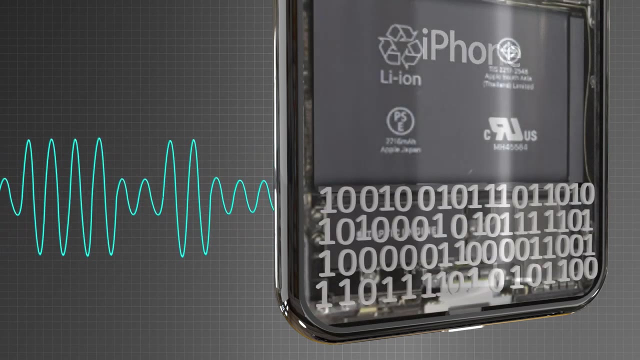 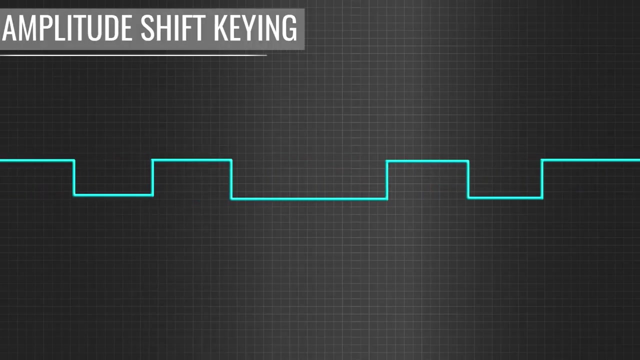 form where the digital signals are either a 1 or a 0.. So let's discuss the digital modulation techniques that are currently used. More specifically, let's see how the digital bit flow is controlled. For example, the digital bit flow is converted to an electromagnetic wave. 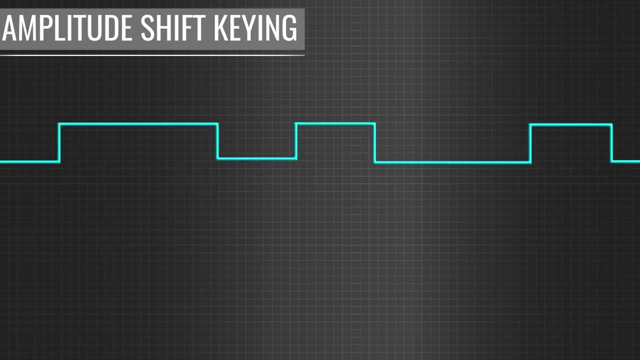 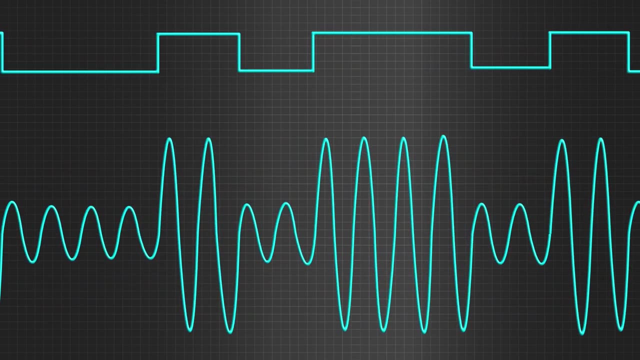 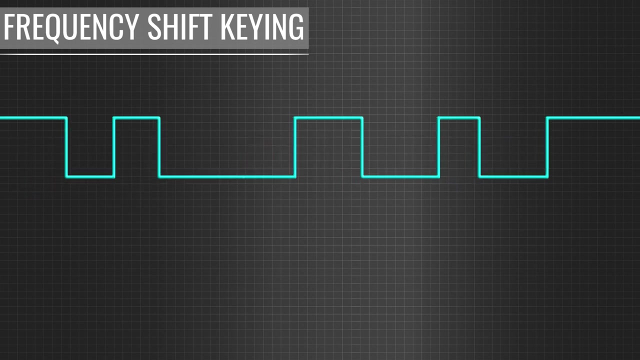 The first digital technique is amplitude shift keying. Here, based on the digital pulses, the amplitude of the carrier signal is adjusted. High amplitude relates to one and low amplitude relates to zero. The next technique is called frequency shift keying. Here, based on the value of digital pulses, the frequency of the carrier signal is adjusted. 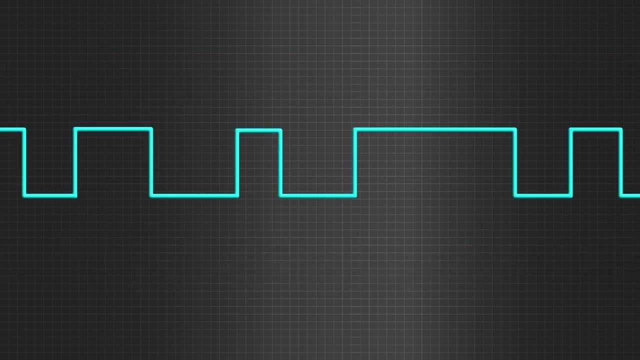 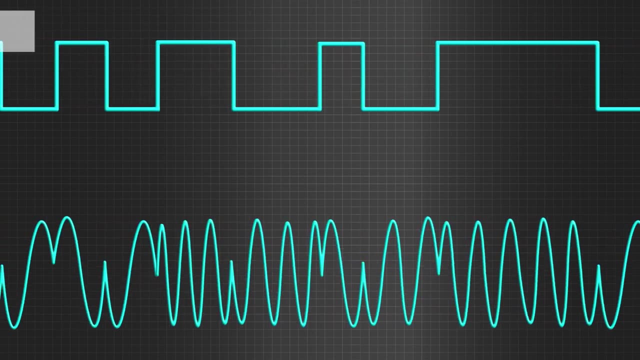 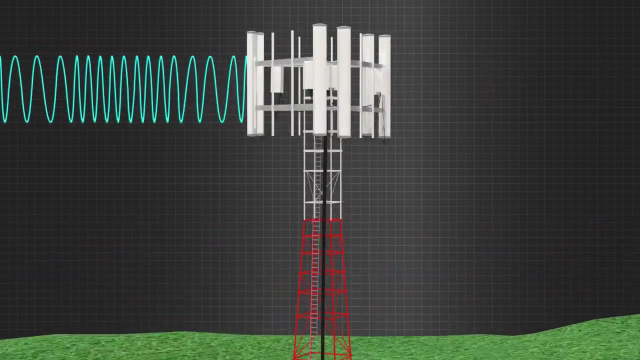 and low frequency relates to zero. the third technique is phase shift keying. here the phase of the carrier signal is changed by 180 degrees when the digital pulse moves from one to zero or zero to one. telecommunications technology is all about increasing data transfer speed and efficiency. but if you use any of the digital modulation techniques explained previously, 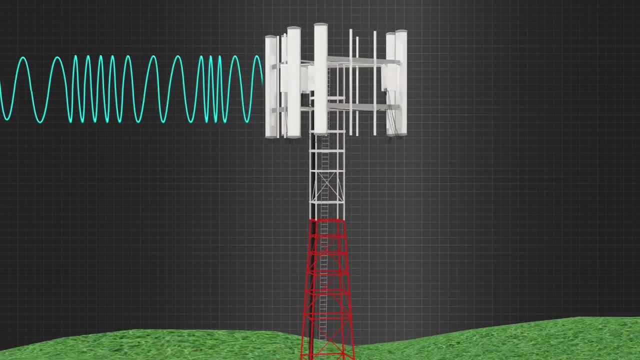 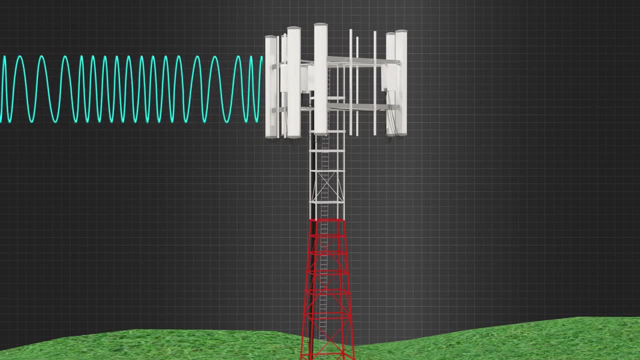 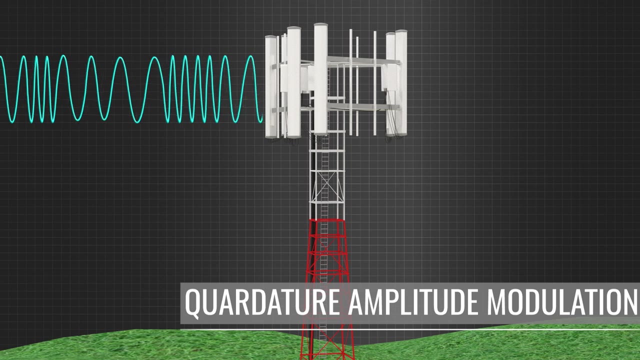 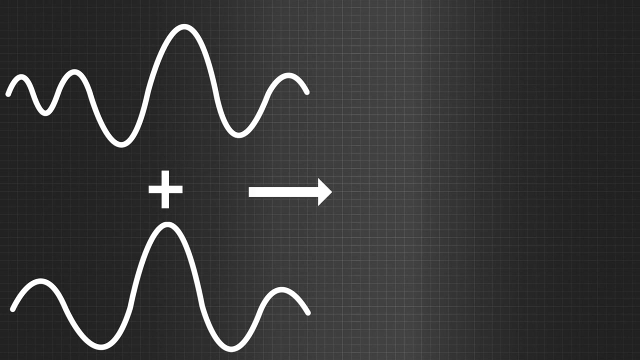 you wouldn't get a high data transfer speed. however, there is a technique in physics which, if you use it, means you can practically send up to six bits of information as a single electromagnetic wave. this technique is known as quadrature amplitude modulation. to understand qam in an easy way, let's take two analog signals. the beauty of qam is that you can. 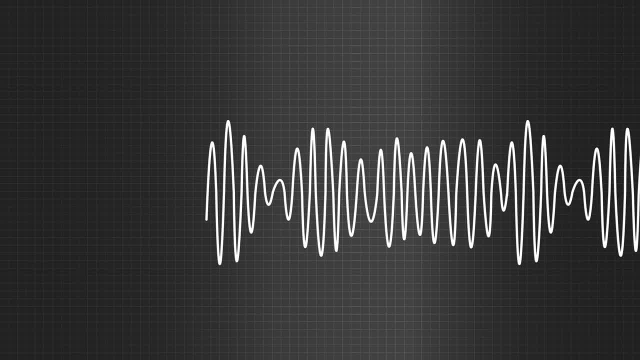 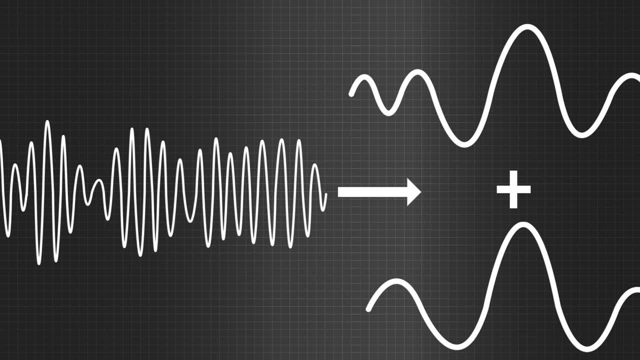 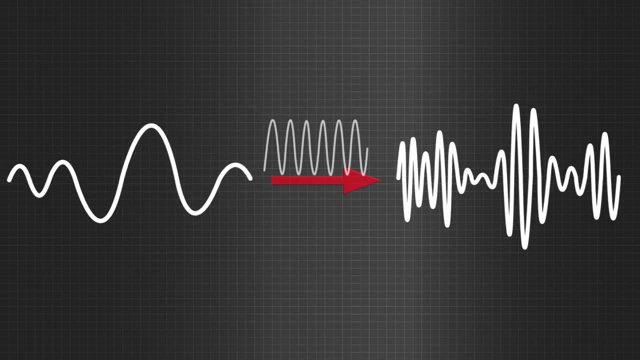 modulate these two different signals as a single signal and then transmit it. then, at the receiver end, you will be able to separate out the original signals, thereby saving bandwidth. let's see how this modulation is done in qam. the first signal is amplitude modulated using a. 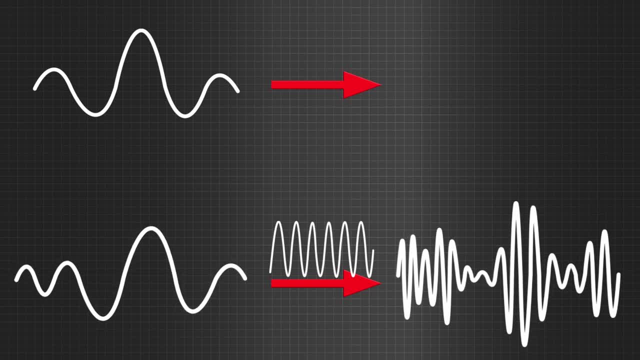 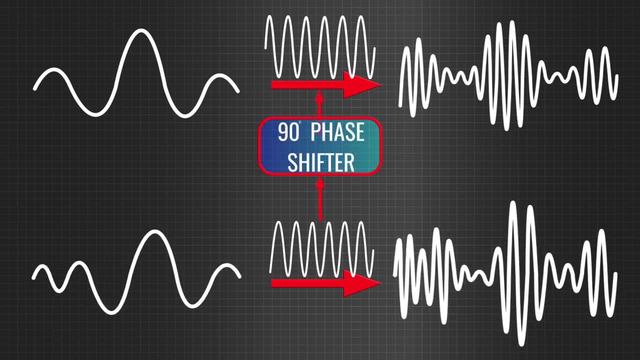 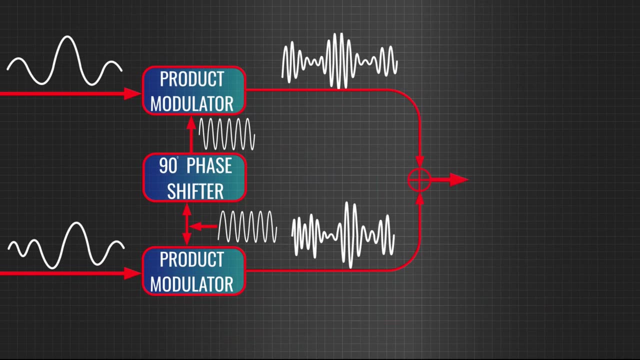 carrier wave as shown. the second signal is also amplitude modulated, with a carrier wave of the same frequency and amplitude, but after giving the carrier signal a 90 degree phase shift. now these two modulated signals are mixed together and form a single signal. we call it a multiplexed 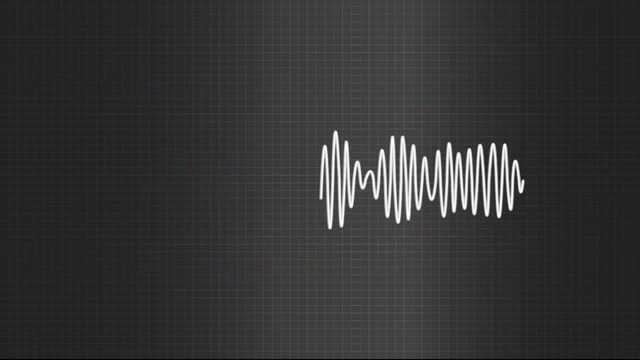 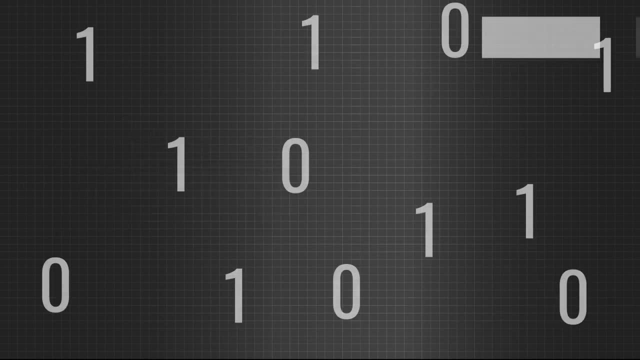 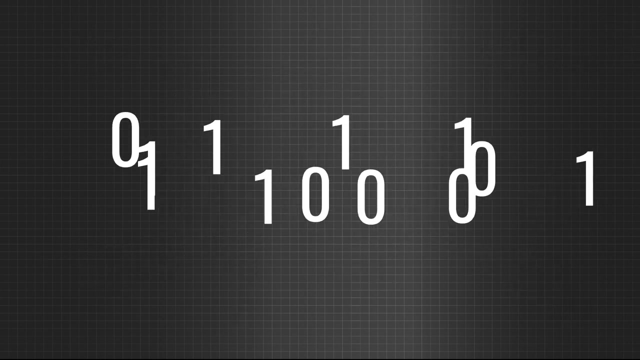 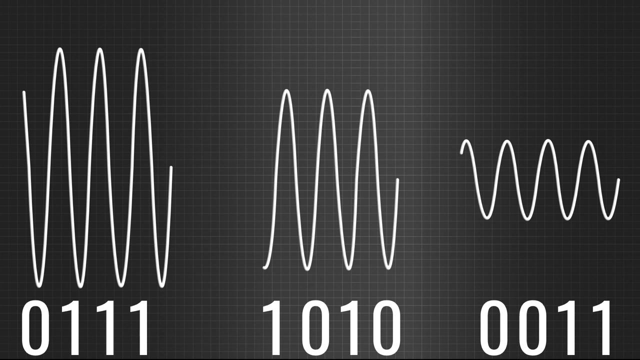 signal. the interesting thing is that on the receiver side, we can easily separate out the original signals from the multiplexed signal. in the case of digital qam, a similar approach is used. here: instead of analog signals, different combinations of bits are added together to produce a multiplexed signal. let's see how a 16 qam works, if you are familiar with. 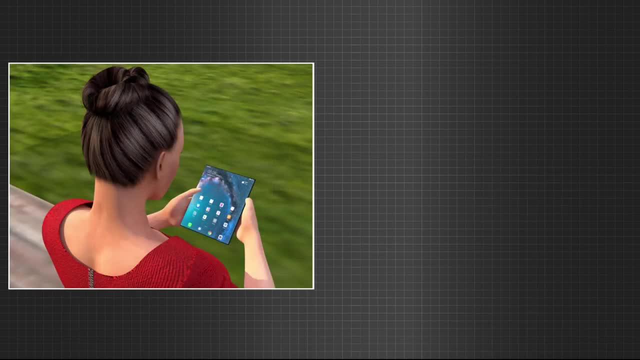 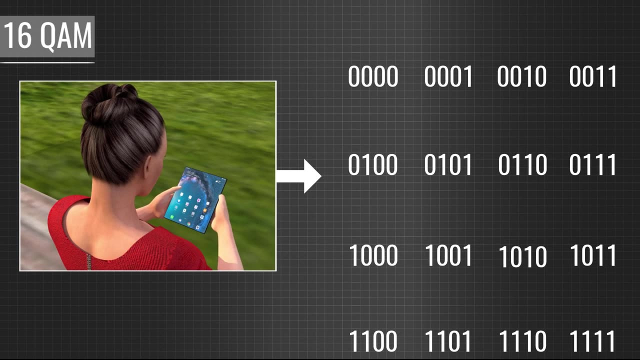 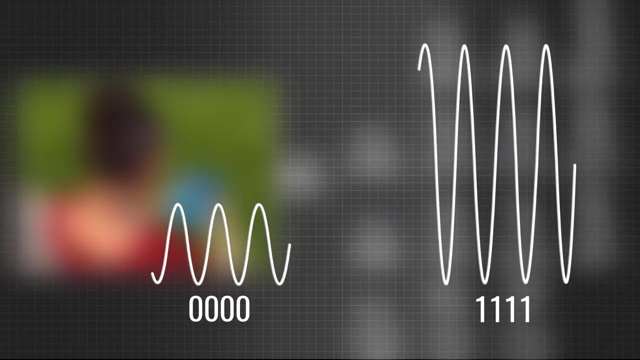 digital technology. you know that any form of data is just a collection of ones and zeros. in 16 qam, we can pack 4 bits together and send it as a single electromagnetic wave based on the values of the 4 bits. this output will have different phase angles and amplitude. 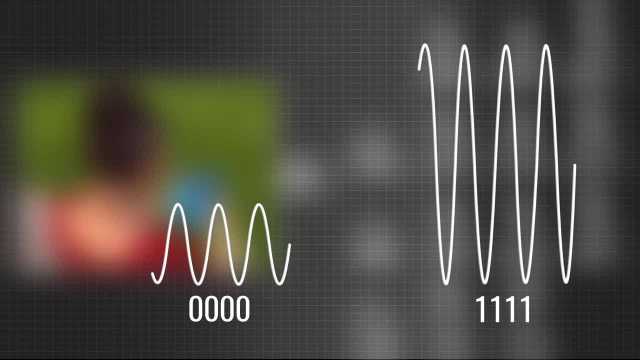 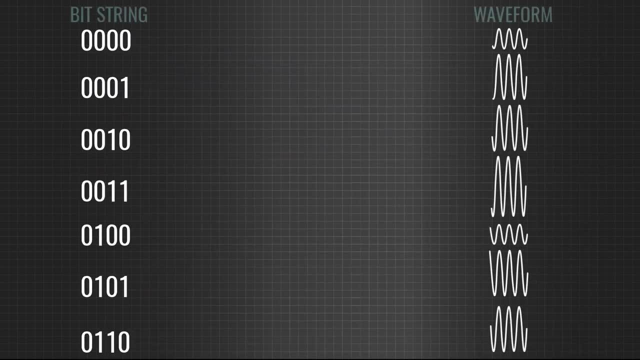 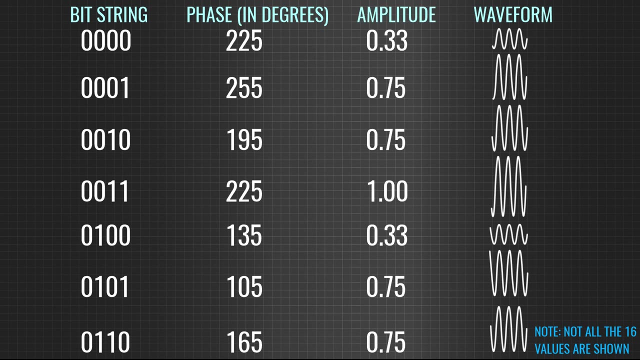 this means the phase, angle and amplitude of the multiplexed signal can completely represent 4 bits of data in 16 qam. such 16-bit values can be represented by adjusting the phase and amplitude of the multiplexed signal, And this single multiplexed signal is then used for the transmission.